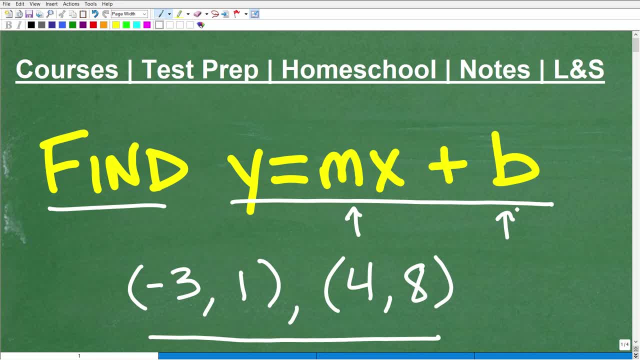 be a pretty easy problem for you. So if you think you can figure this out, go ahead and put your answer into the comment section. I'm going to show you the correct answer in just one moment And then, of course, I'm going to walk through the solution here step by step. But before we get, 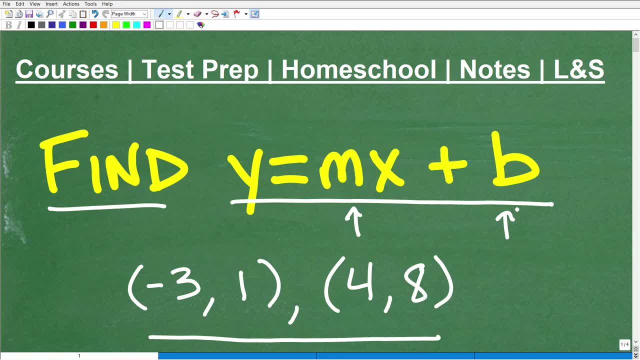 started. let me quickly introduce myself. My name is John. I'm the founder of TC Math Academy. I'm also a middle and high school math teacher. I have been teaching math for decades and I want to help you be as successful as possible in mathematics. So if you need help in your current 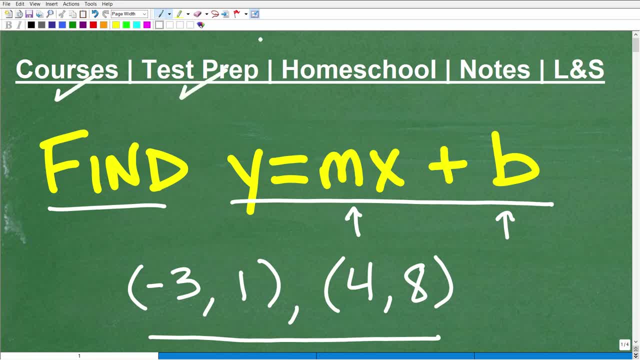 math course or maybe some sort of special test, something like the GED, SAT, a teacher certification exam, or, if you're a math teacher, you can help me out with that. So I'm going to walk through your home schooling mathematics. Check out my math help program. I'm going to leave a link to it in. 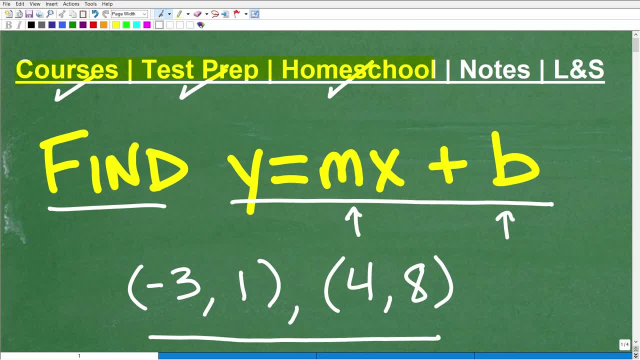 the description of this video. I promise it will make learning math much, much easier. Also, I'm going to leave links to my math notes in the description as well. You absolutely need to be taking great notes to be successful in math. So if your notes are so-so, you can use my notes in. 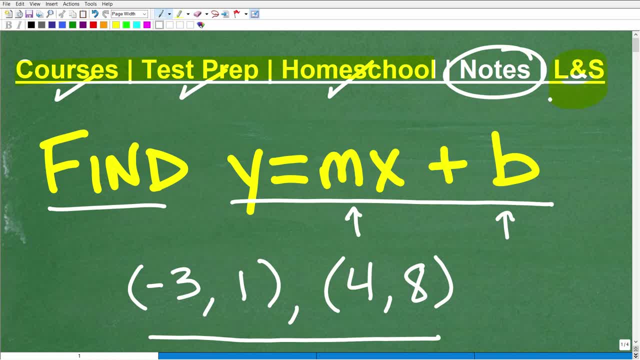 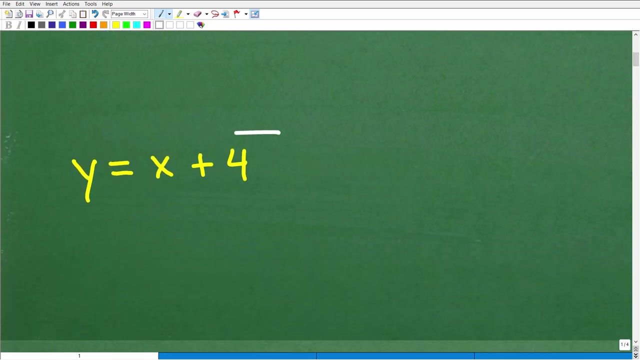 the meantime, as you improve your notes, And if this video helps you out, don't forget to like and subscribe, as that definitely helps me out. So let's go ahead and take a look at the answer here. It is: y equals x plus four. All right, So 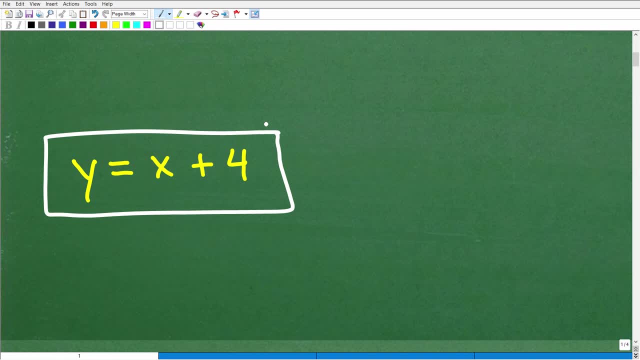 how did you do? Well, hopefully you got this right. Matter of fact, if you're able to do this, let's go ahead and give you a nice little happy face and a plus a 100% And a few stars, so you can tell your friends and family that you know how to find the equation of 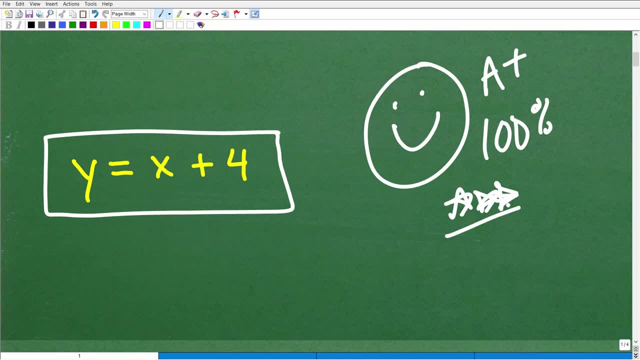 a line given two points. I'm pretty sure they would be very impressed by that. So don't forget to tell people that you know how to do some algebra. OK, now, this is some algebra, because of course there is a lot to know in algebra- but linear equations, graphing lines, finding the 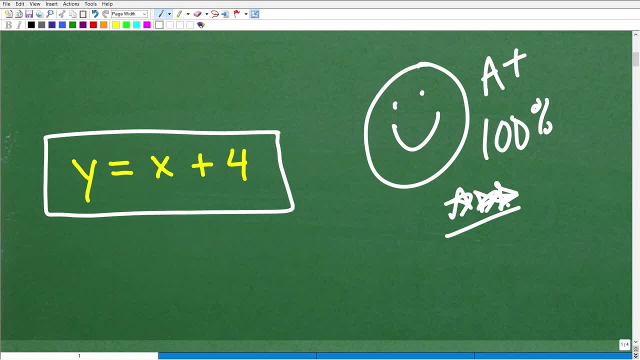 equations of lines is. that's hugely important for all of you out there that are studying courses like pre-algebra algebra one, certainly algebra Two. OK, so let's go and get into this problem Now. there's a lot of different variations to this. 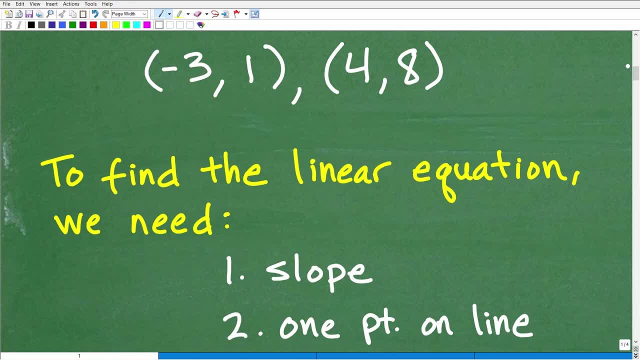 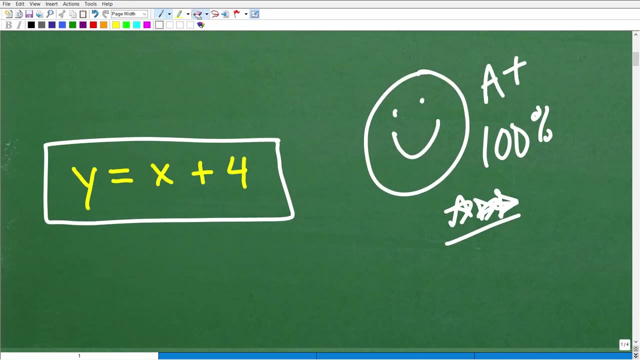 type of problem which is find the equation of a line or write the equation of a line or find the linear equation, given some information. Now, if you think about it, here we have one point and another point. OK, so on the x- y plane, here let me kind of back up and we'll just kind of erase. 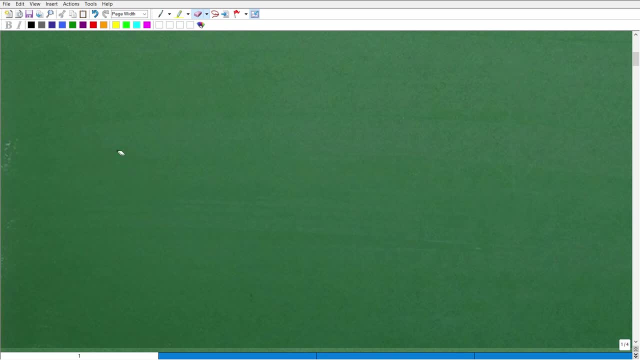 all this here for a second. Now I just want to kind of give you a basic visualization of what's going on here, Right? So here is a lovely x- y axis. So if I have this point and let's say another point, I have two points and that's what we have in this particular 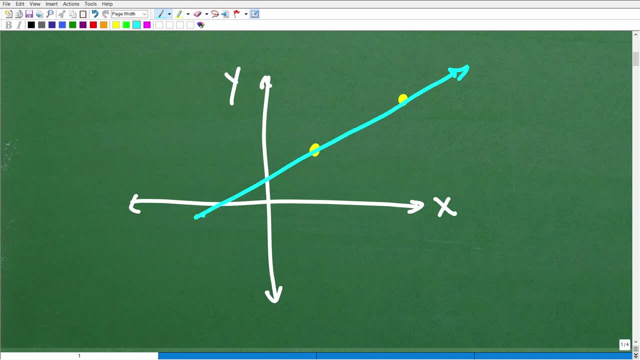 problem. Well, I can certainly graph the line, OK, because I have two points. OK, but that's not the question. The question is: hey, give me the equation of this line. ie and y equals mx plus b four. So we have two points and we want to find the equation of the line. So we have two points. 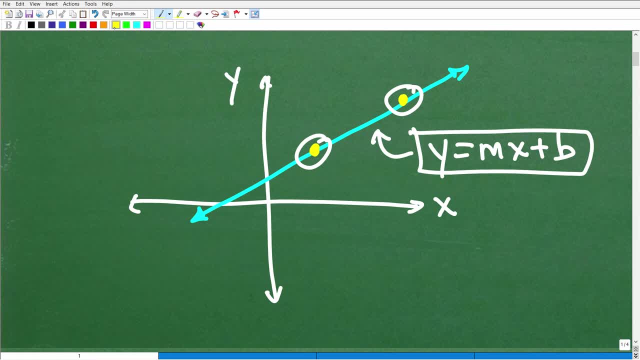 on this line. Now, this type of problem typically comes after once you've learned how to graph linear equations. So hopefully you know something about the slope, how to find the slope, how to graph lines, et cetera, et cetera. So just kind of graphically, this is kind of what's going on. 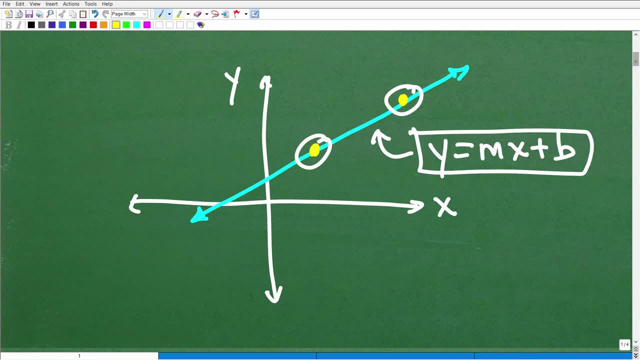 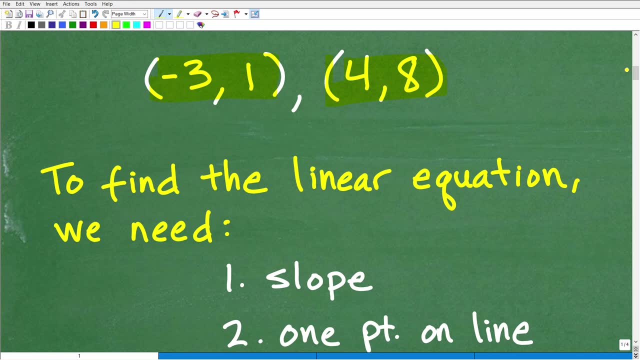 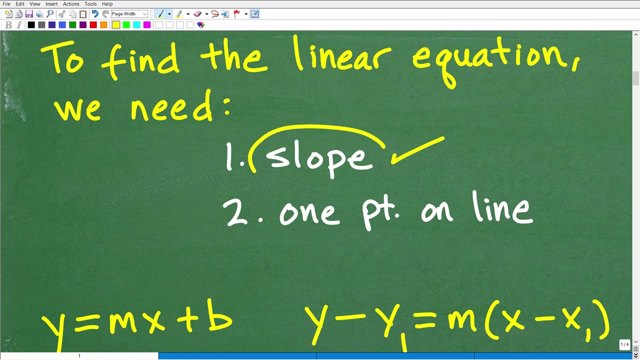 We want to find the equation of the line, And here we have two points that are on this line. So how do we do this? Well, when you want to find a linear equation or find the equation to any line, you always need two pieces of information. We need the slope- OK, we need the slope of that line. 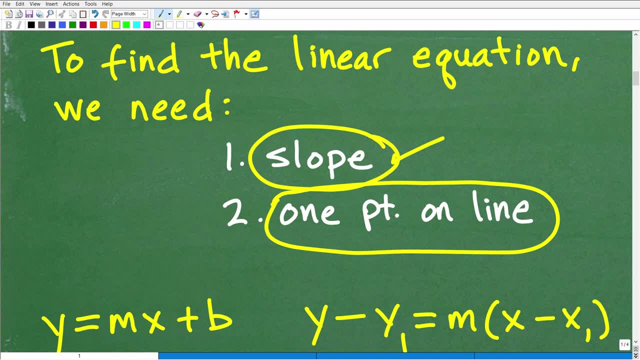 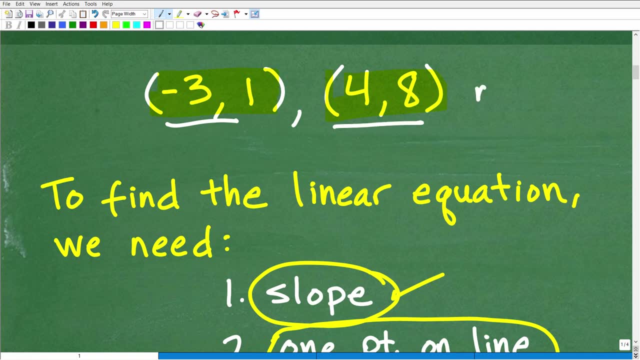 and we need at least one point that's on that line. So, with this particular problem, what we have is two points that are on that line, but we do not have the slope. But is that a problem? No, because if we have these two points, we can calculate the slope And then, once we have the 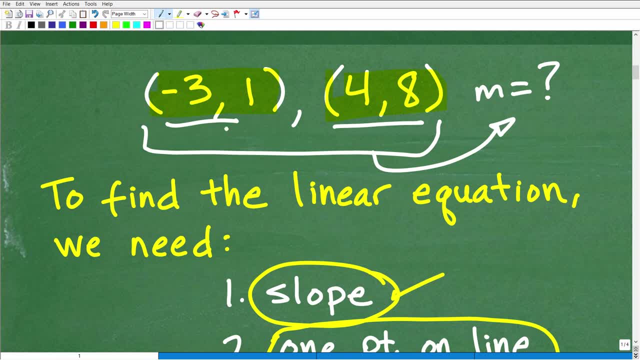 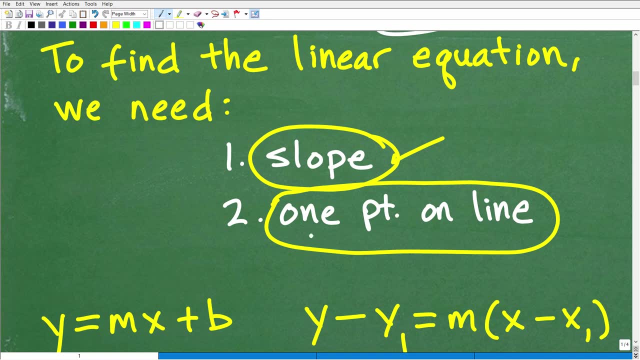 slope. we can either use this point or this Point to answer the question, But this is the basic information that we need. We need the slope of the line. At least one point is on the line Now. once we have that information, we can use one. 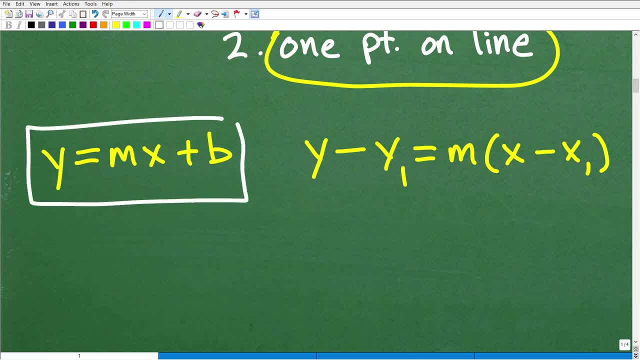 or two formulas. We can use Y equals MX plus B, which is the slope intercept. This is the Y intercept and this is the slope. You can use the Y equals MX plus B formula to actually find the equation of the line, But I'm going to suggest that you get 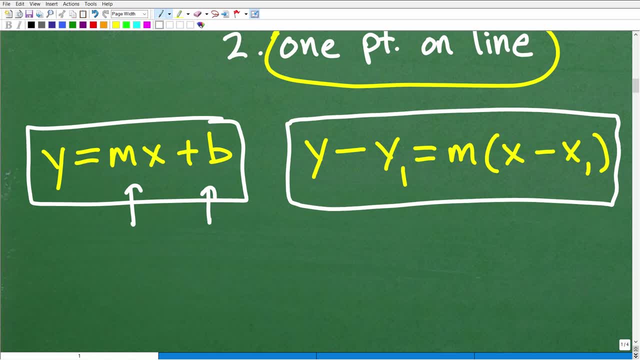 really familiar and, as a preference, OK, like. in other words, if you're thinking about OK, what formula should I use to find the equation of lines, I'm going to suggest using the point slope formula. So this is the point slope formula, right there, And I'll explain this because this is 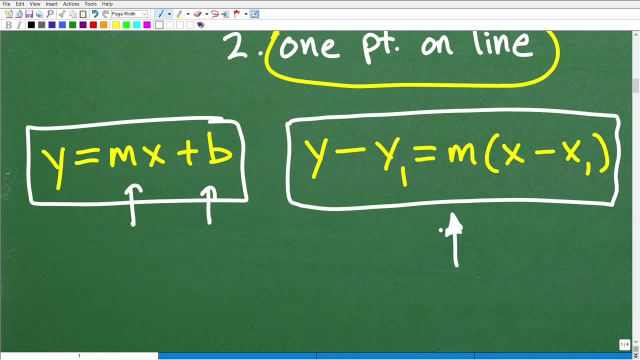 in a second, because this is the formula I'm going to use to find the equation of the slide. But again, you could use the slope intercept formula. But here's the deal: Once we use the point slope formula, we're going to be able to find the equation of the line. So this is the point slope. 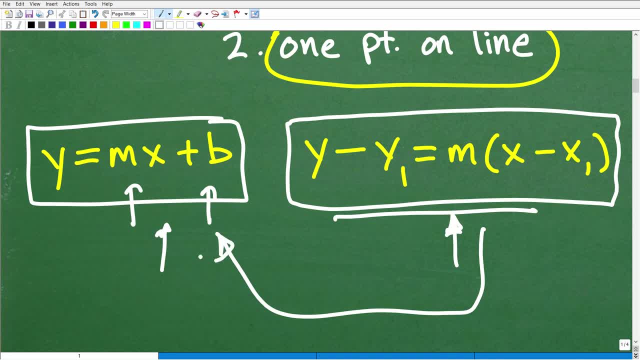 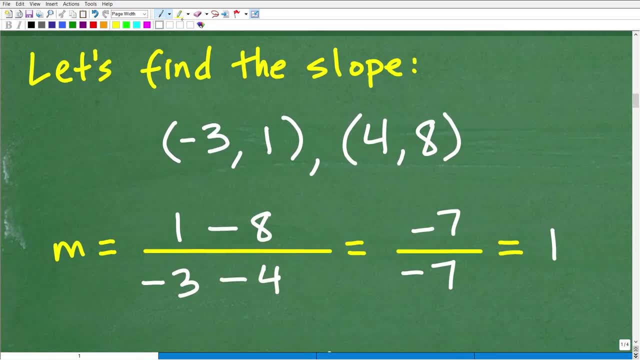 formula, Our final answer will be: in: Y equals MX plus B form. OK, so let's go and get into this right now. All right, So the first thing is we need to find the slope of this particular line. So we know that we have two points on this line. So how do we find the slope? So remember, 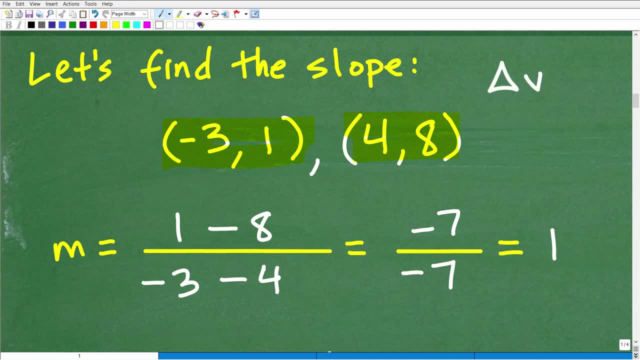 the slope is the rise over the run. So it's the change of Y's over the change of X's. In other words, we have to subtract the Y's and then we have to put that That's. that'll be our numerator. 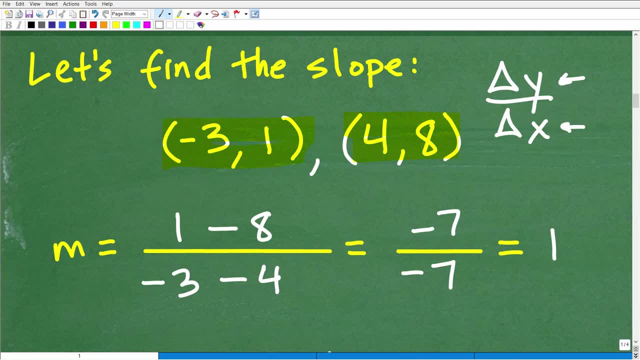 And the differences of the X will be our denominator. There's a lot of different ways to write the slope, But basically, if you can't calculate the slope, you need to go back and review how to calculate the slope. You can find all this information that I'm talking about here. 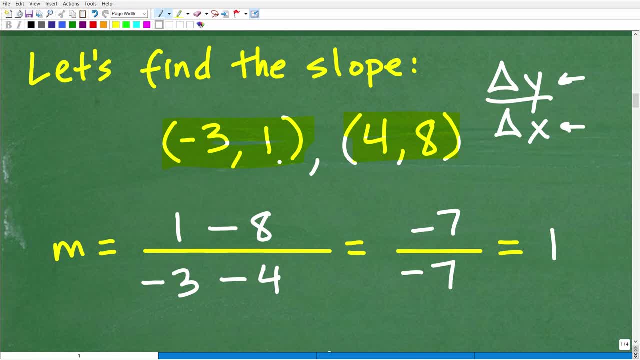 in my pre-algebra and algebra one course, even my algebra two course. All right, So what we need to do? the biggest error that students make when calculating the slope is they mix things up. In other words, I'm going to give you a suggestion. 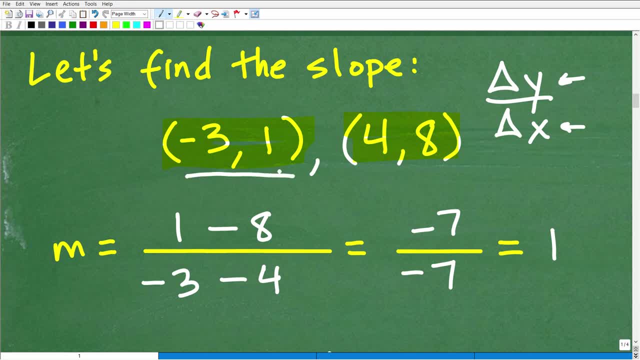 Take a point to start with. I like to underline a coordinate like this, So we're going to take this one. OK, this is our Y, So let's just kind of really take our time here with our slope, because some of you out there might be confused. So this is an X- Y coordinate, and this is an X- Y coordinate. 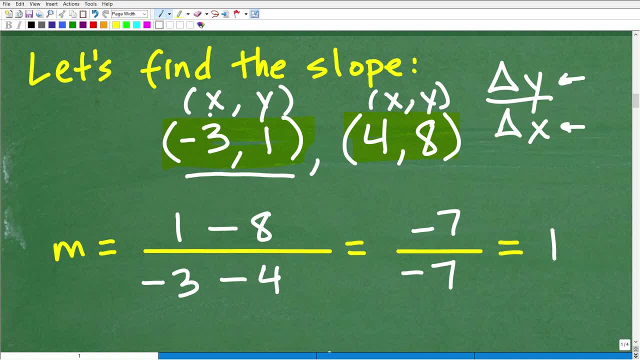 right there. So for this point, Y is one and this point X is negative three, And in this point Y is eight And this point X is four. So what we need to do is subtract the Y's, That's the change in the Y's. So do we go one minus eight or eight minus one? 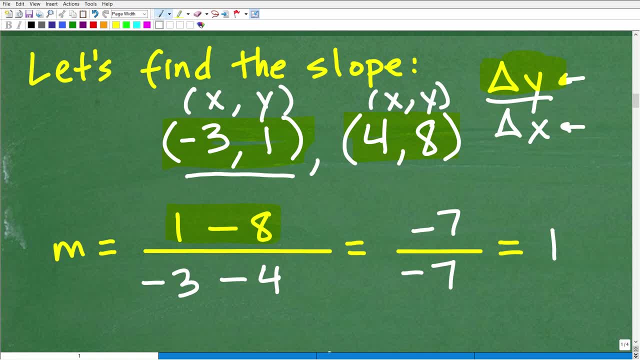 It doesn't make a difference. OK, but I'm going to suggest, if you're going to go one minus eight, just underline the point you're going to start with, because this can? this has a huge impact on your final answer. So one minus eight is going to be what? one plus negative eight, or? 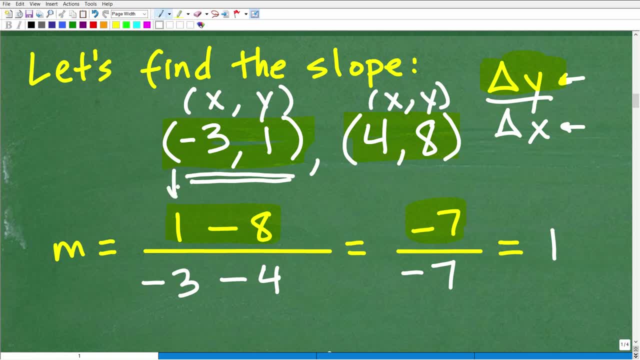 negative seven Now, because I started with one. OK, my right here I did one minus eight. When I subtract the Y's I must start with the X coordinate for this Y. So in other words, I started with this. points information one. So when I subtract the X's down here, I'm sorry, 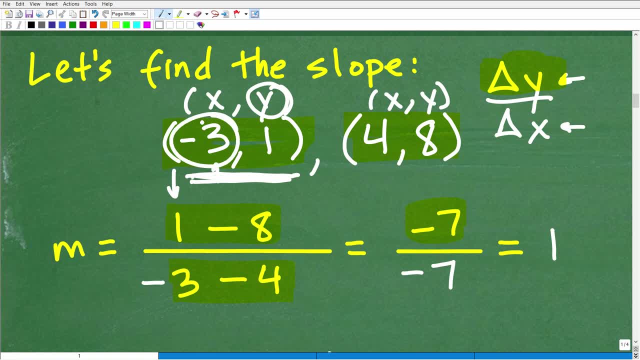 I think I said Y's. When I subtract the X's, I must start with the negative three. A lot of students get confused. I'm like, oh, that's four minus a minus three. No, no, no, If you start with. 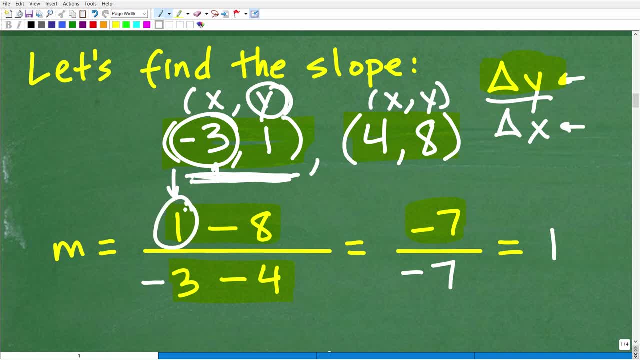 this points information here we have to have. if we have one as our Y, we have to have our negative three as our X. So now we're going to have negative three Minus four. OK, this coordinate right there. So negative three minus four. So that would be. 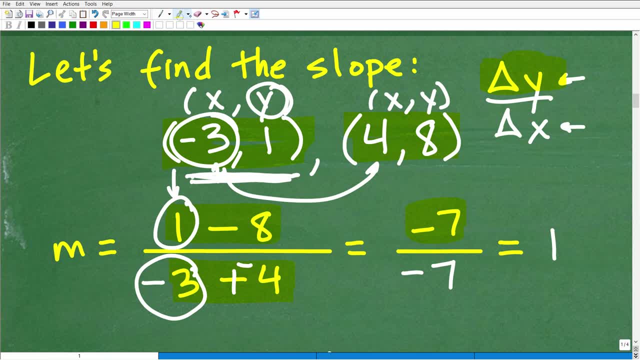 negative three plus a negative four, which is negative seven. So we have negative seven or negative seven, which is a positive one. So I think oftentimes when students are trying to find the equations of lines, they make a lot of mistake with the slope. OK, so if this is something that's. 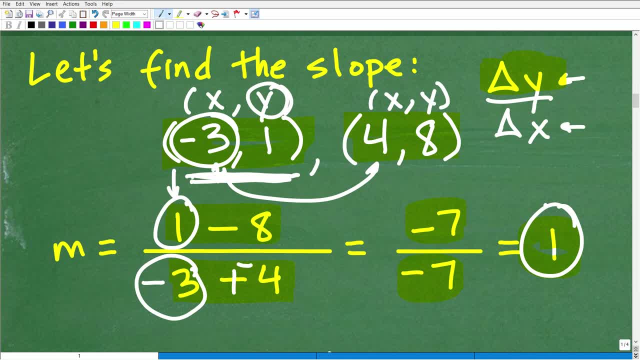 been bothering you and if you're not, like sure, why are you getting these type of problems wrong? It's likely you could be calculating the slope incorrectly. So I have all sorts of different additional videos on my YouTube channel about the slope and graphing lines et cetera. But again, 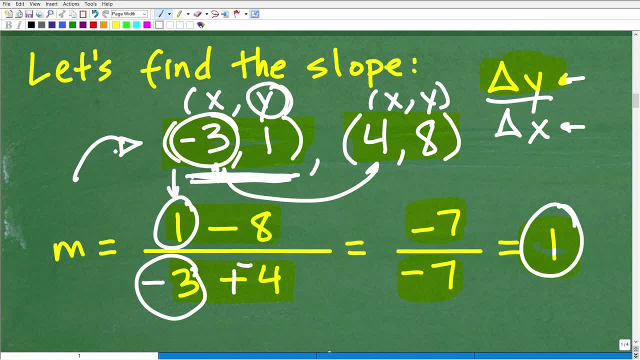 I'm going to suggest you just kind of get into my formal instruction and, like my algebra course, You can learn everything you need to know. All right, So, anyways, the bottom line is that we do have the slope. Now. it is one, All right. So the information we have is: we have two points. 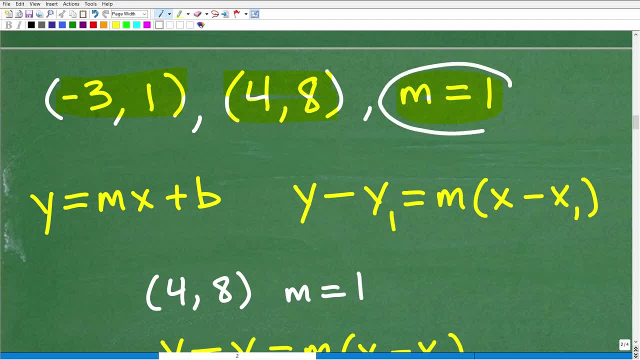 So remember, what we need is the slope, for sure. OK, that's non-negotiable. And we need one point that is on the line Here. we have two points, So you could just select either point. You can get the correct answer using this point or this point, So just try to identify the one. that's a little. 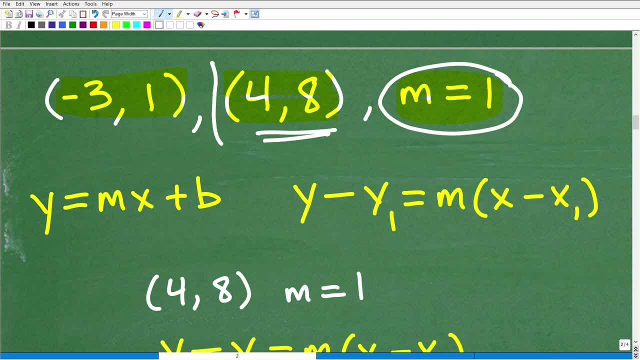 bit easier to work with. I'm just going to go ahead and use four- eight. So now we're basically kind of change the question. Let's find the equation of a line that has a slope of one that passes through the point Four eight. That line will also pass through the point Negative three one. All right, So now if 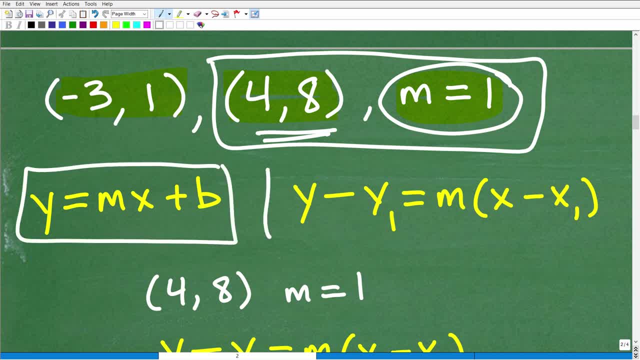 you understand that. again, remember, we have two options: We can use the slope intercept formula or the point slope formula. We're going to use the point slope formula right now, OK, so how does this work? Well, here at the point slope formula, let me just go and circle the things we're going. 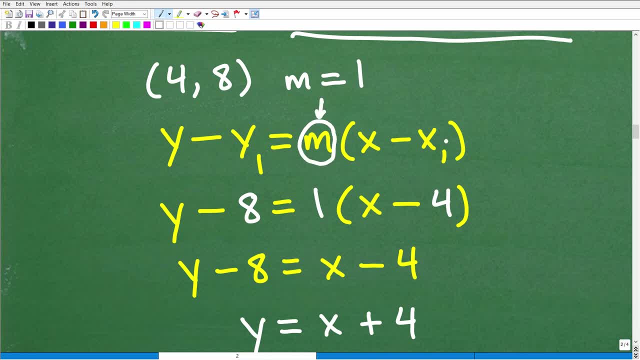 to plug in. So for M, we're going to plug in the slope X one, We're going to plug in our X value On our coordinate that we're going to be using in this case. that's going to be four, And then eight. 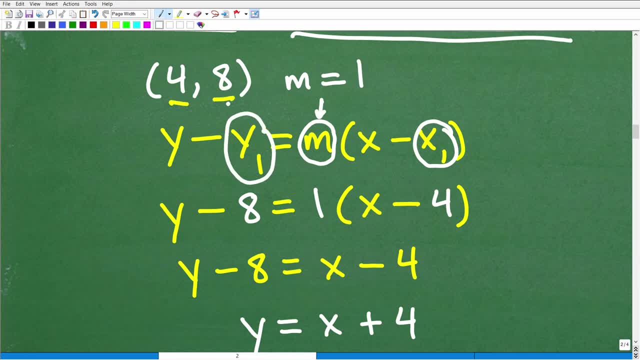 is our Y coordinate, So this Y one, we're going to plug in that eight. OK, remember, when you're dealing with a coordinate it's always X, Y In our case. here our point is four, eight, So these: 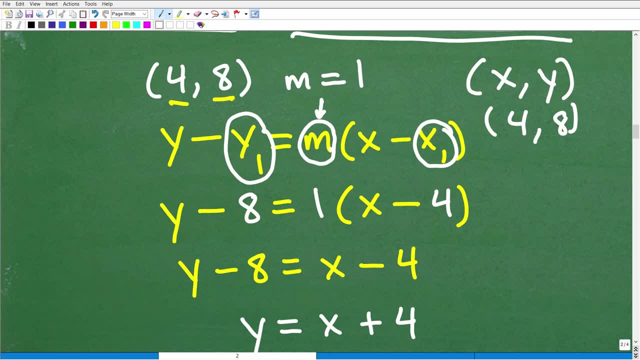 Y ones and X ones. these are the plug in values that you're going to use for the point slope formula. OK, so let's go ahead and plug in those respective values. You can see here- I already did: minus eight is equal to one, which of course is the slope times X minus four, which is again. 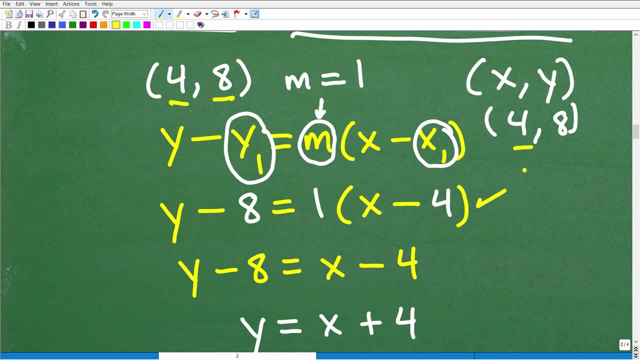 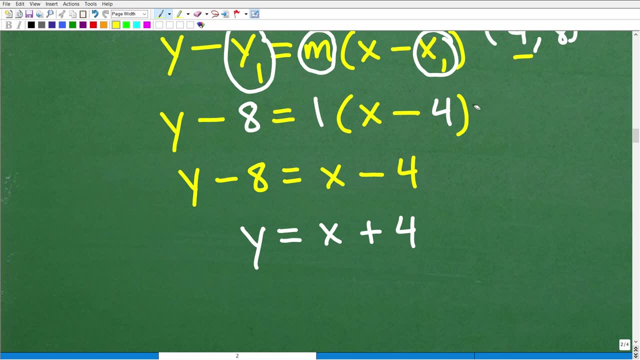 our X coordinate for our point. All right. So at this stage all we need to do is basically solve for Y. So what you want to do is just apply the distributive property. So that's going to be one times X, which is X, And that's going to be one times that four negative four. So that's. 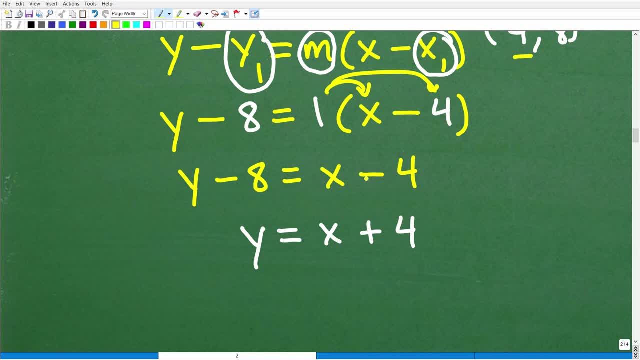 negative four. So you have: Y minus eight is equal to X minus four. So what we need to do to solve for Y is simply add eight to both sides of the equation. So we have negative four plus eight, which of course is a positive four, And this is our final.